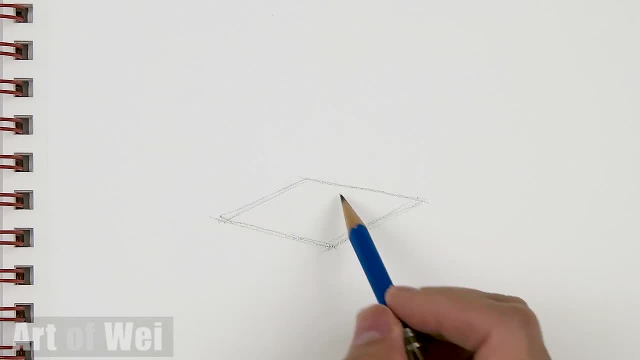 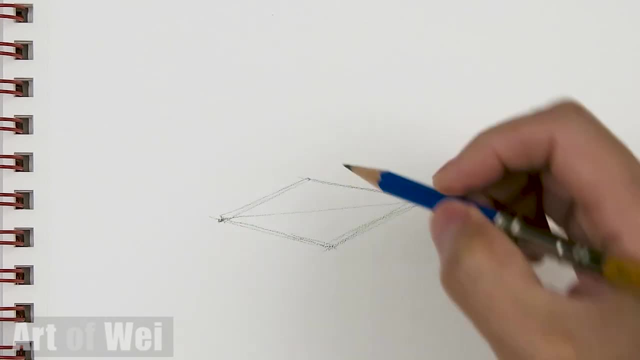 and in order to find the tip, we're gonna have to find the center of this base. So to find the center, just draw a line corner to corner, and then where it intersects, that's gonna be your corner, I mean your center. and then, from this, 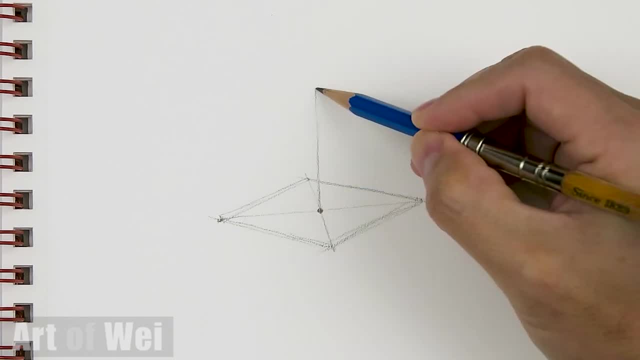 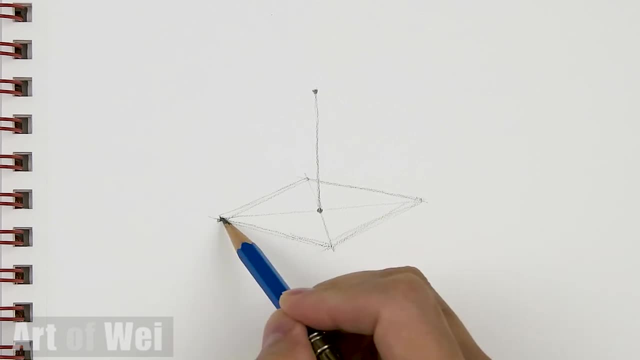 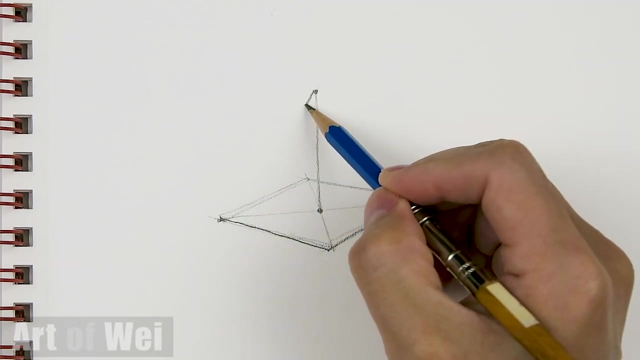 center. we'll just go straight up. I'm just gonna draw it this high, Okay, Maybe I should make the lines a little bit darker, Okay, so from this tip, it's really simple. Now we're just gonna come down, connect to the corners and 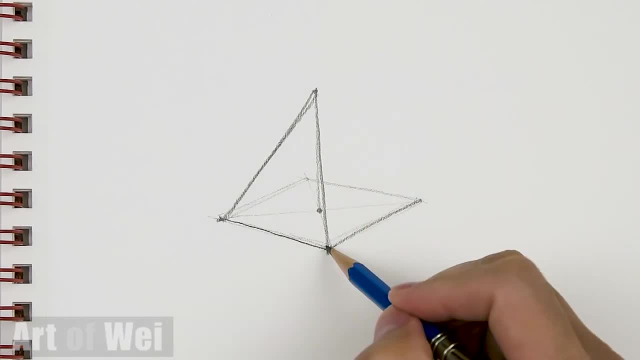 sometimes this line kind of goes over. Hopefully you guys can still see that: Okay, so that's the pyramid and this one right here. this- this is gonna be the back right, So we won't see that. Okay, so that's the pyramid and this one right here. this- this is gonna be the back right, So we won't see that. 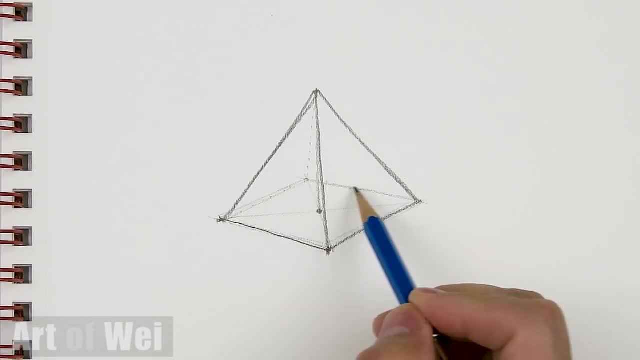 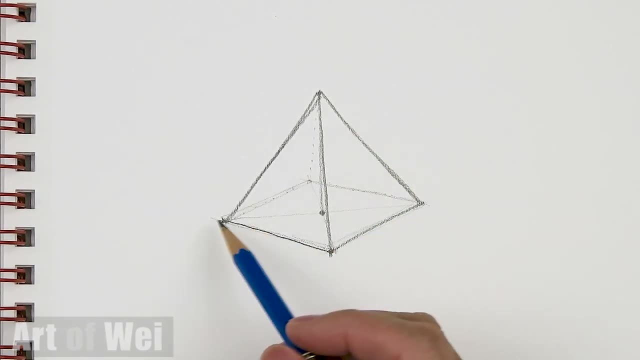 Actually, this was gonna be the back too, so this should be a dotted line, Alright. so that's pretty much it for this. Any kind of pyramid you want to draw, just draw on the base, find the center and then just go straight up and then. 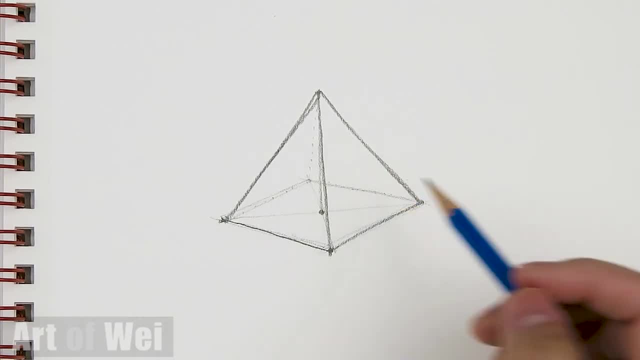 connect to that. Alright, so once we have this, let's have a little fun and let's shade it How we can add in a little bit of shading, because without the shading, you know, things kind of get lost, right. You don't know, you know what. 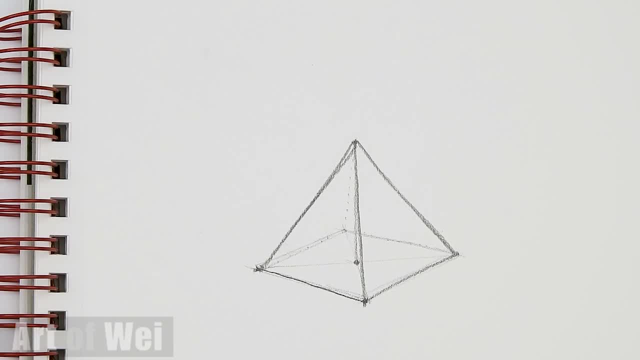 these lines are for Alright. so now we're done. Now let's draw a light source for for this. so we got, we can shade it and add in the shadow, And this is kind of the same way how we add shadow to a lot of basic. 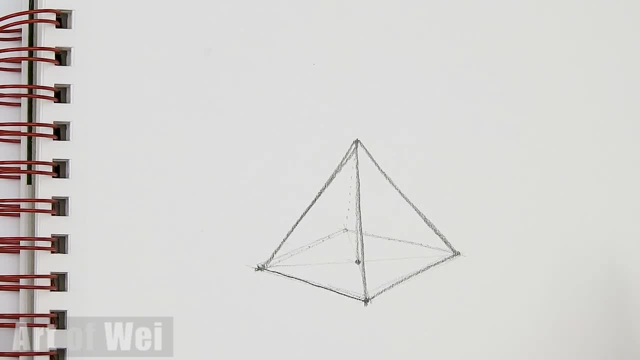 shapes. We kind of learned this in perspective class a long time ago. Okay, and so let's just say, we're gonna have a light source up here somewhere, right, We're gonna draw a little lamp so we can draw in. let's say, this is the floor we're. 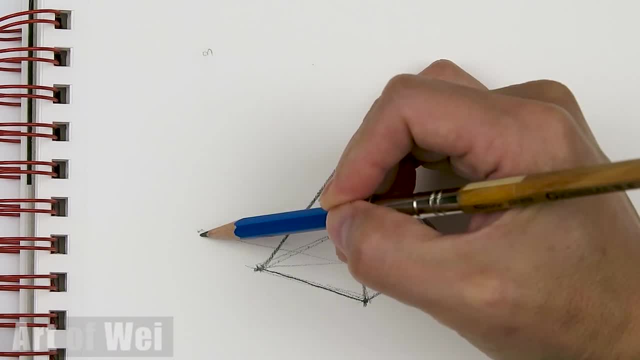 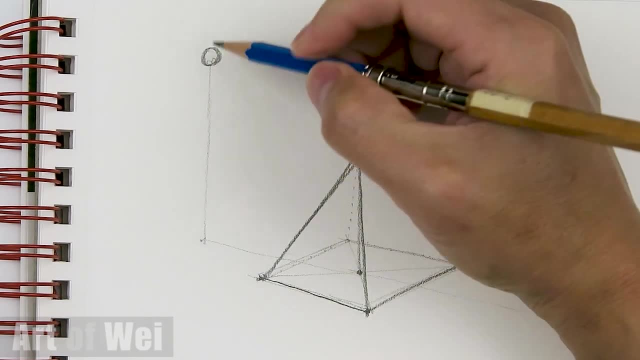 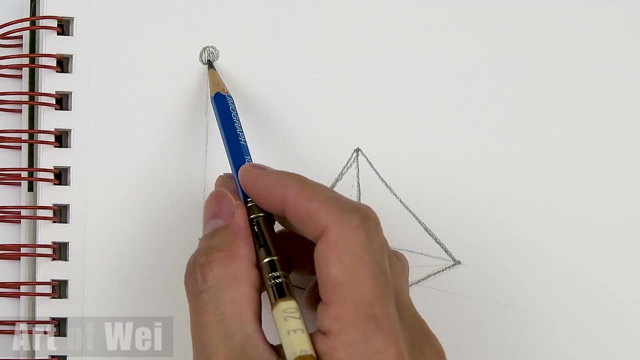 just trying to visualize this line here, and then from here we'll go up, So this will be a lamp or whatever it is. So here's the light source. Okay, so now to find the shadow of this is actually quite simple. We'll just continue on with. 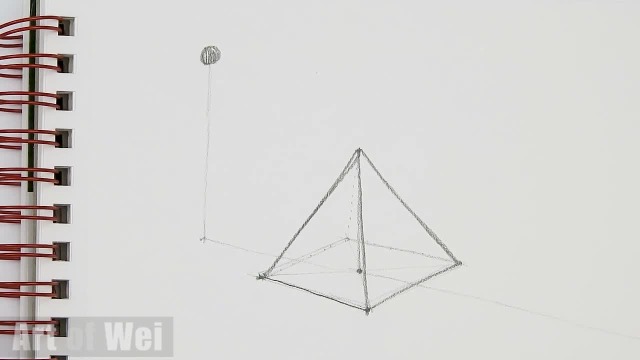 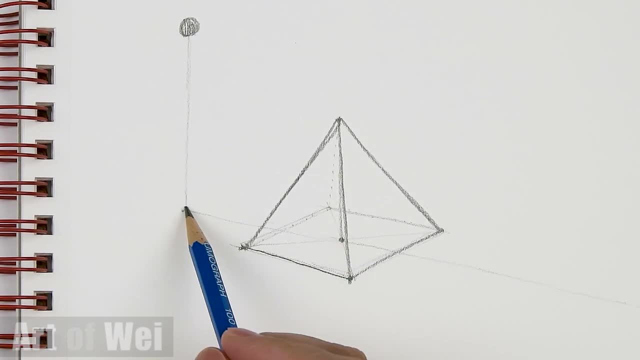 this line right here We go all the way out, because we're trying to find this point here where it's going to cast all the way to the floor. Okay, so we have one line, here's the floor, and then, from the light source, we're just going to hit the. 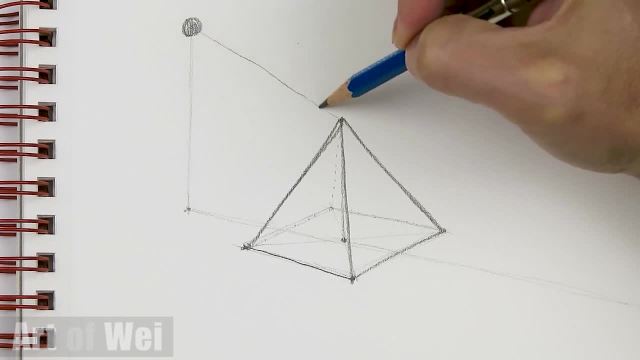 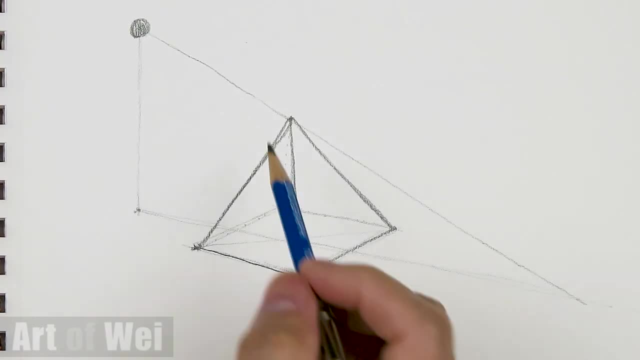 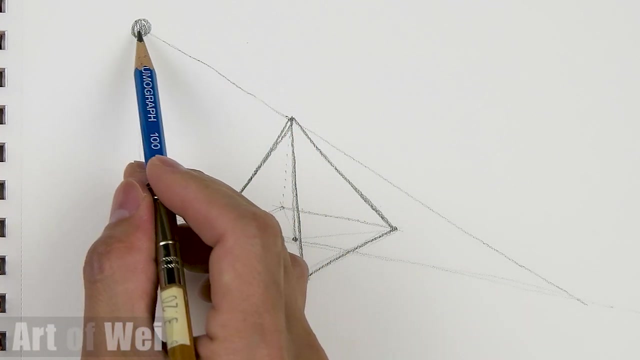 this corner and we're gonna keep extending it until we intersect with this line here on the floor. Okay, so I'm just free handing everything, but the idea is the same, even though it's not, you know that accurate. So it's just gonna come across, okay, from the light source to the tip, to the corner here. So 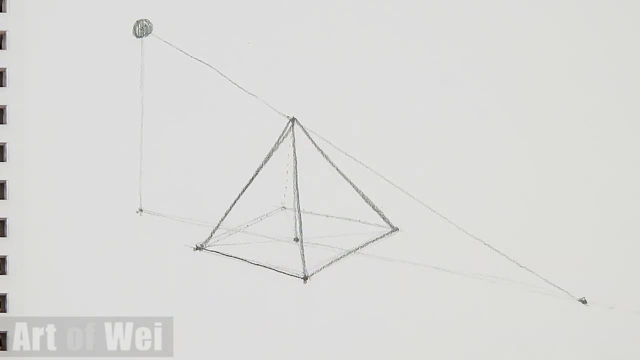 this is this point, right here. This is shadow point, right here. Okay, so that's the tip. That's the tip. So now, in order to connect these, we're just going to go through these and this one's very simple, So we'll just go here, connect to here. 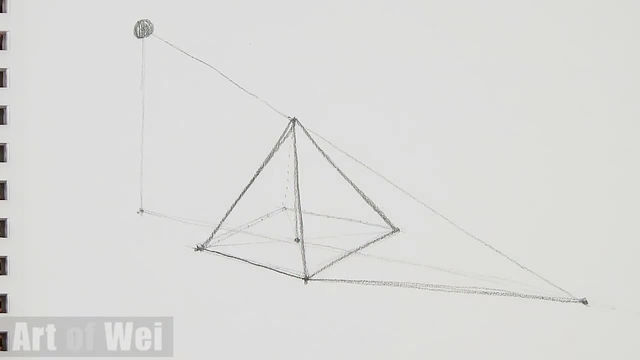 Alright, so this edge is basically this edge right here, and then, of course, this edge right here from this point will connect to that. Okay, so this face right here is basically this face in shadow, So let me shade this in. So this will be all. 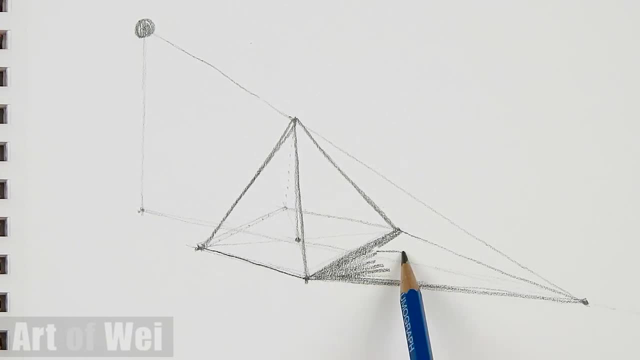 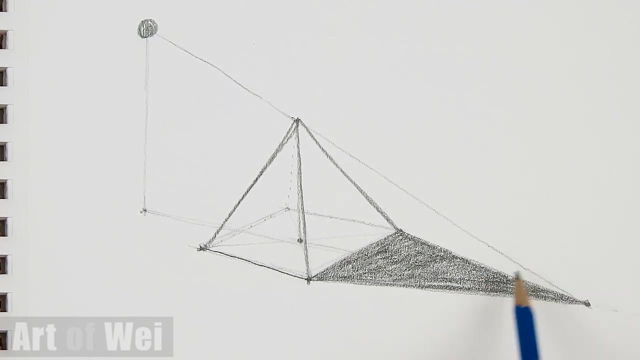 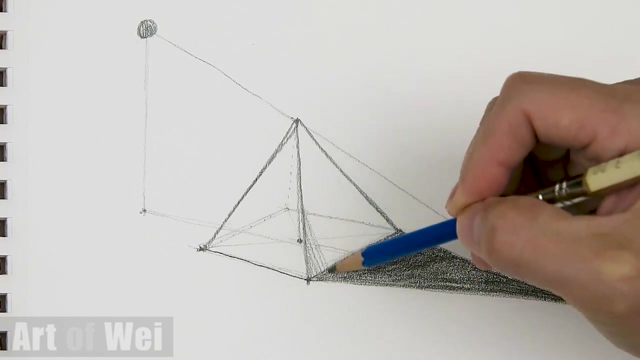 black. I'm just using a 4B right here. Let's make this tip nice and sharp. Okay, so that's the shadow, and then, of course, now we have to shade this part, because this one's going to be in the shade. And then, once we shade this, we're going to actually be 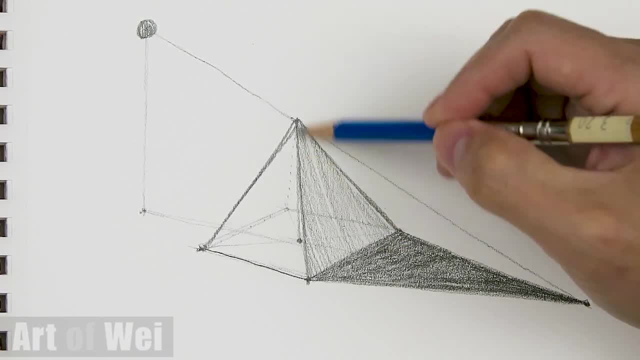 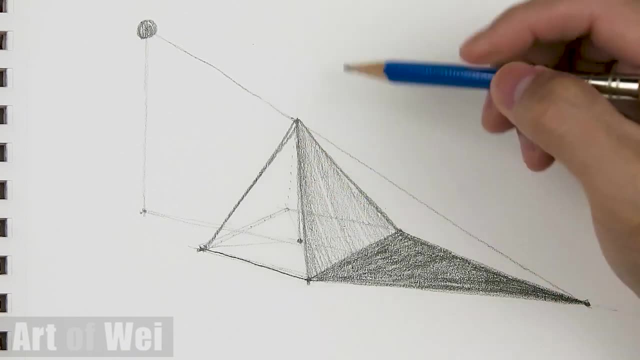 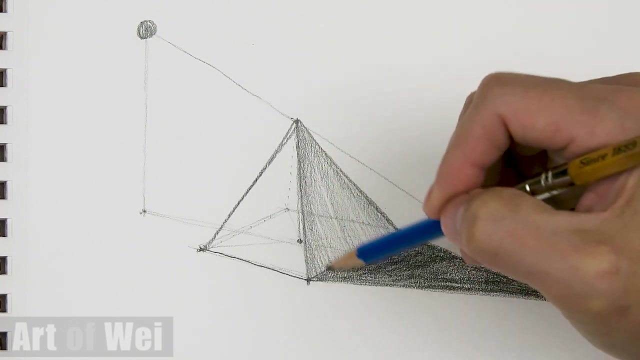 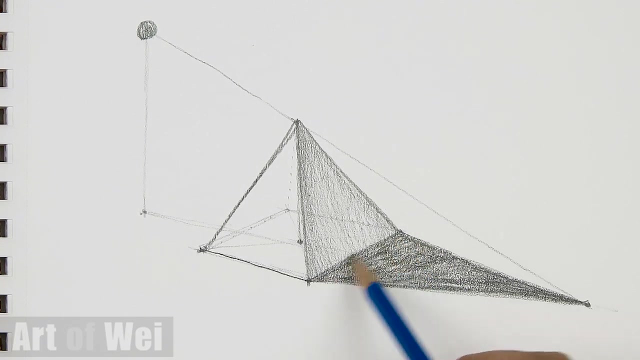 able to visualize this shape a lot better. I'm gonna make this edge right here a little bit darker, just to exaggerate and give it a little bit more contrast, so it just makes it a little bit more dynamic. Okay, and if you like, let's see if this is the shadow right here. See all this white? 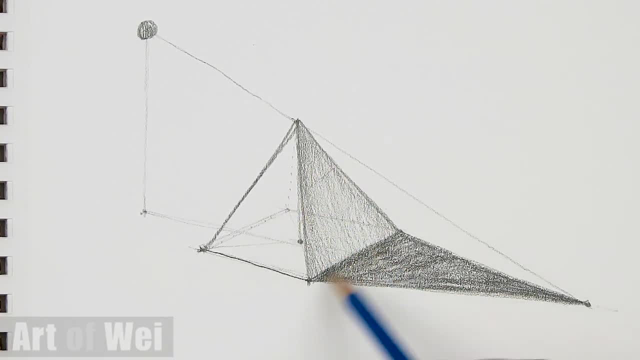 space is gonna bounce back up, right. so this part would be a little bit wider and this part should be a little bit darker, because you're not getting as much bounce light. So right here I'm just kind of nitpicking and trying to make things a little bit more realistic. 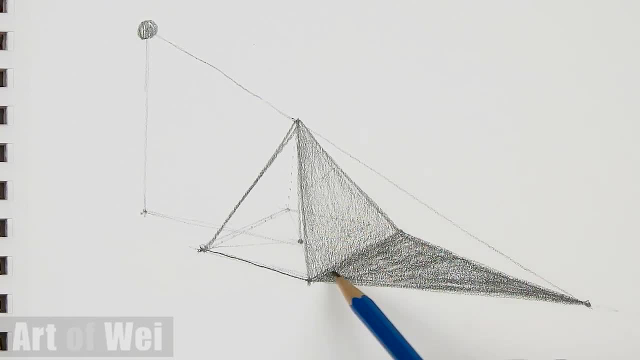 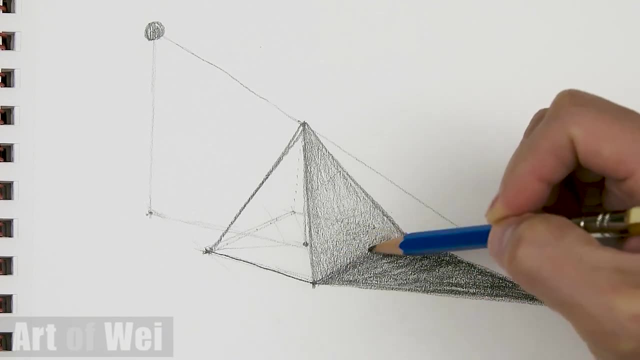 I'm going to make this edge a little bit darker. I'm going to make this edge a little bit darker. I'm going to make this edge a little bit darker, All right, so then this side it's darker, and then this one. actually, you know. 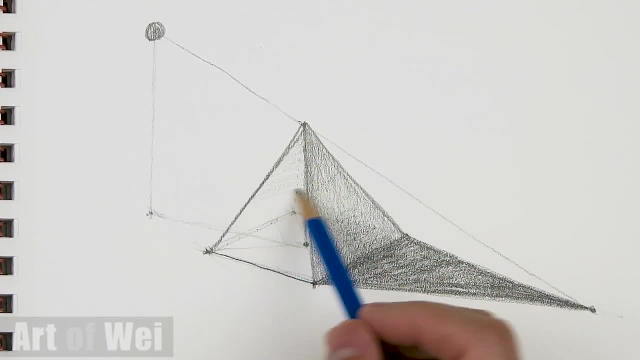 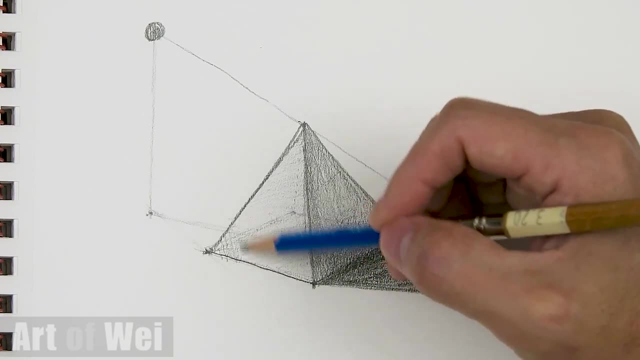 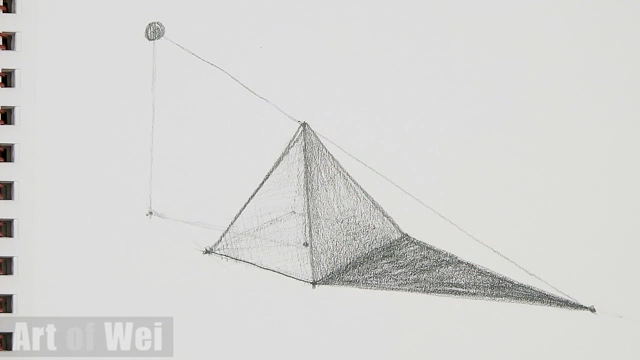 because we're not facing the, the light source, directly. so this should be a shade to this part, should be darkened, that. but okay, get the idea, okay. so that's how you can draw a pyramid. so let's see, let's draw another one on right here. 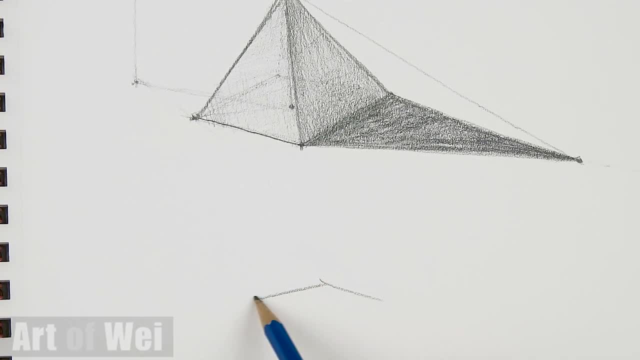 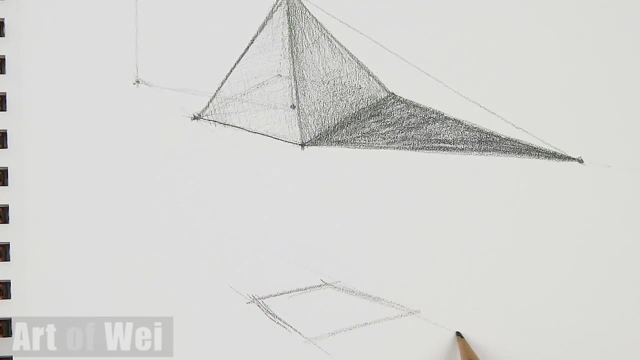 right here. let's see, let's try, try it this way. like extreme, a little bit more creasement there, all those parts. so I'm gonna give it a little bit more transfer right extreme, a little bit more extreme. Madonna de dark yellow, all those perspective here down the middle here, alright, the. 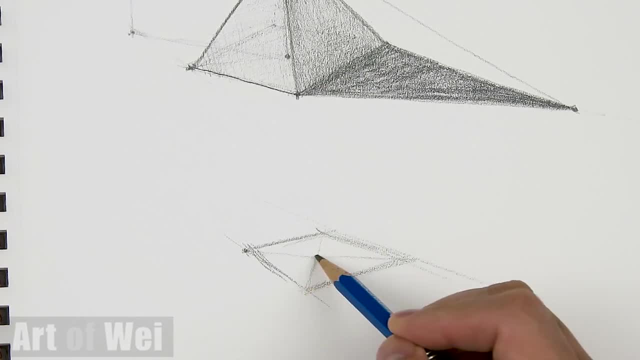 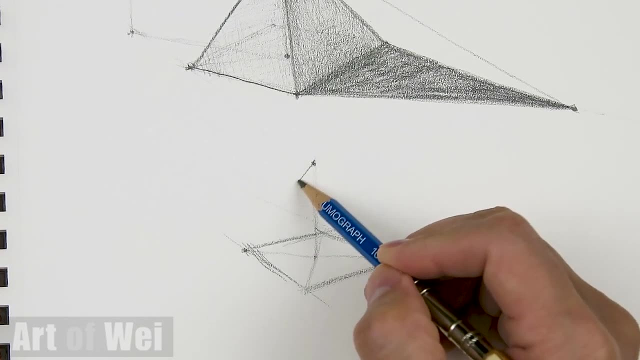 okay, so we're gonna find a center corner. okay, so we're gonna find a center corner. the center would just go up. there's the. the center would just go up. there's the tip, however tall you want to make it. and tip, however tall you want to make it, and. 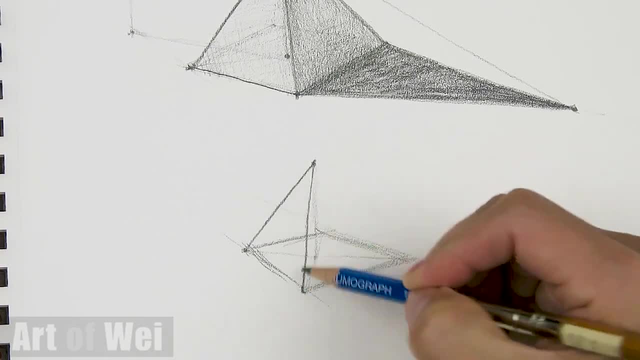 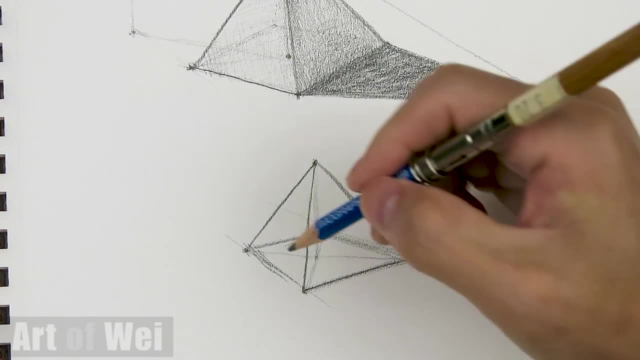 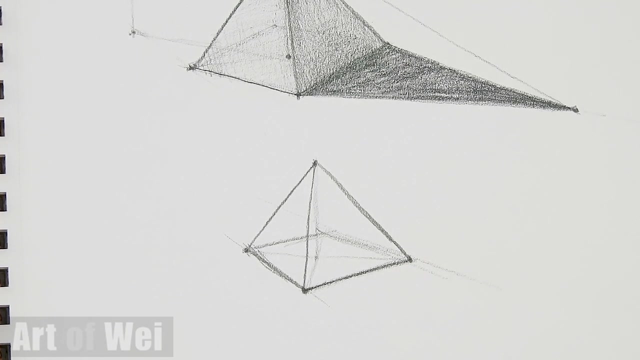 then from here, just connect to that, connect to all the cornersALRIONAL. Okay, this one looks a little bit more dynamic because of the extra perspective, more extreme perspective, All right, and then for the light source: if you want to draw it, let's put it here. 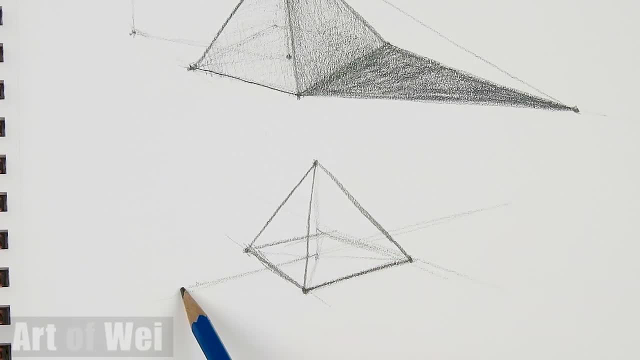 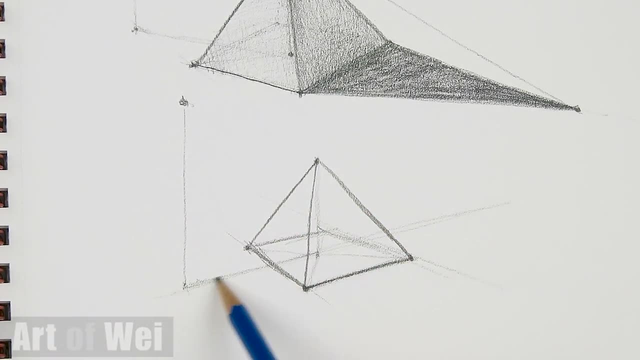 Let's see which way. All right, let's put it out here. Here's the floor, Here's the lamp. We'll go up here. Okay, so extend this line on the floor wherever it is, and then we'll just connect this.